hey everybody, my name is Julian and today I'm going to be talking about color theory. this is a really important topic for any artist or graphic designer- anything surrounding art. you need to know color theory, and I also get asked a lot of questions about color theory and things to do. 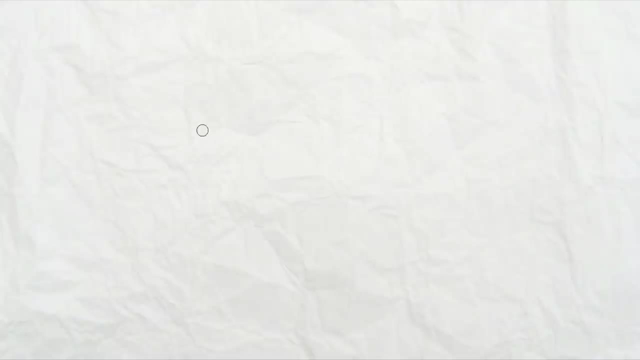 with colors a lot, so I thought I might as well make a video for you all. so I'm going to start with hue. this is pretty straightforward and it's pretty easy to understand. hue is essentially what color the color is. so if I draw a little graph here, I want to draw red in the middle. I will 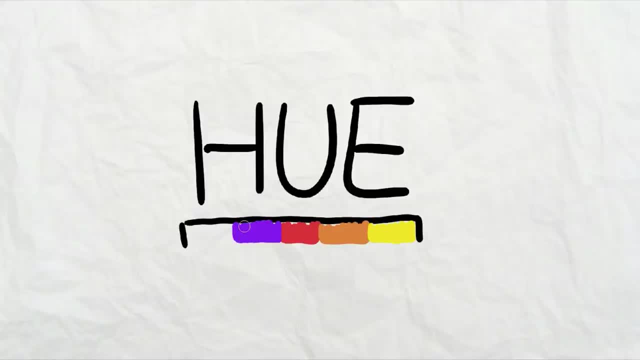 draw orange, yellow will draw purple next to the red and then pink. you can see this color is basically changing and yeah, pink should be next to red, but let's ignore that. so essentially, hue is just what color it is. so if we have a color red here and we duplicate this and 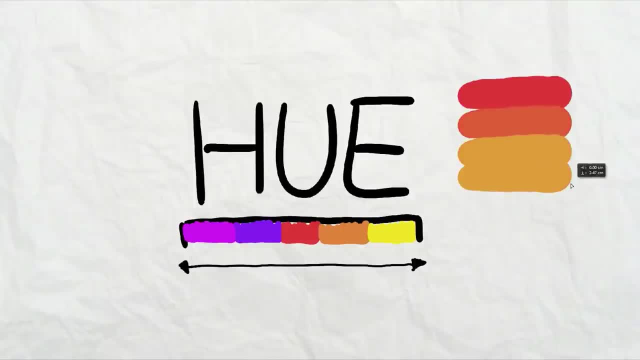 we change it. we've just shifted the hue from a red to an orange, and then we've shifted the hue to the orange to a yellow, and then we shifted the hue from a yellow to a green, and so on. it's basically just what color you have selected. there's not much more to it. the next is saturation. 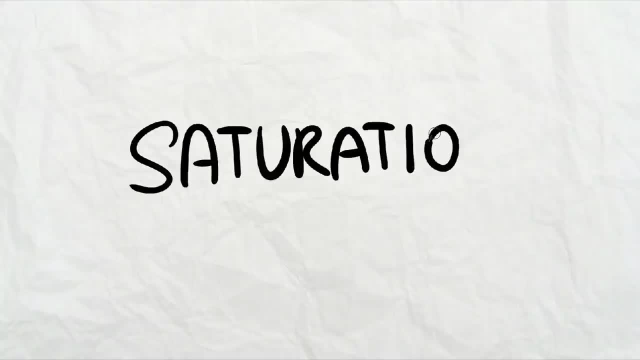 so this is a word you're probably going to see a lot if you work with Photoshop or any sort of digital program, and you'll probably hear it a lot too in the art world. this is essentially the intensity of the color. this doesn't change how light or dark the color it is, it doesn't change. 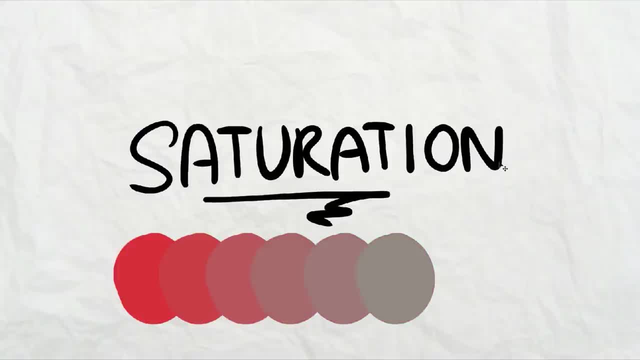 what color is. it just changes how intense that actual color is. so, like you can see on my screen, I've got a bunch of dots. the left hand dot is a hundred percent saturated. the right hand dot is zero percent saturated. so no saturation of a color, is just gray, and this applies for any color. so you 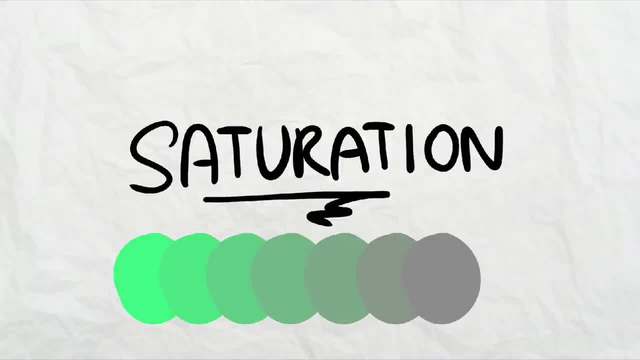 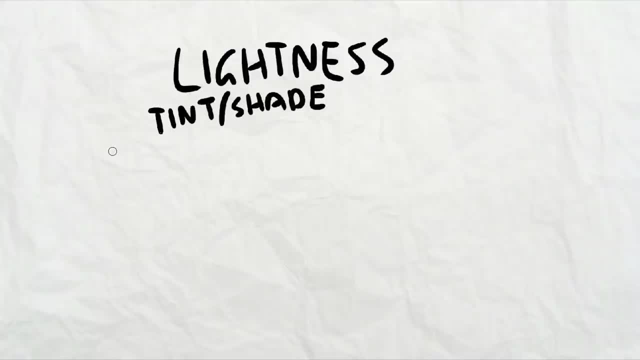 into tints and shades. so this is basically how bright or darker color is. this doesn't affect the hue or the saturation or anything like that. it's basically just adding white or black into the color. so if I sort of draw some little rectangles here, you can see I'm sort of making them lighter. 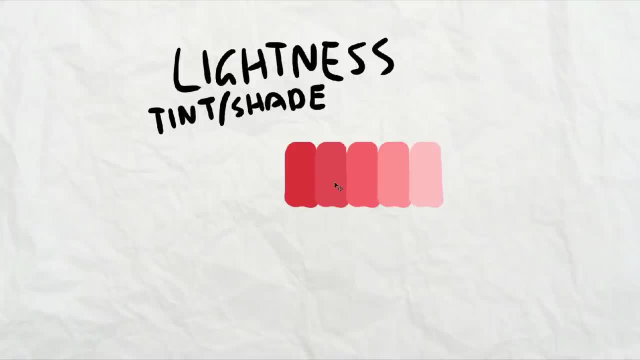 and lighter. so they're basically tints and then I'll make some more and I'll make it darker and darker and these are some shades, so you can see the darkest colors, sort of like a dark brown, but then the light color is basically like a pink and it still has a lot of color. it's just very light. 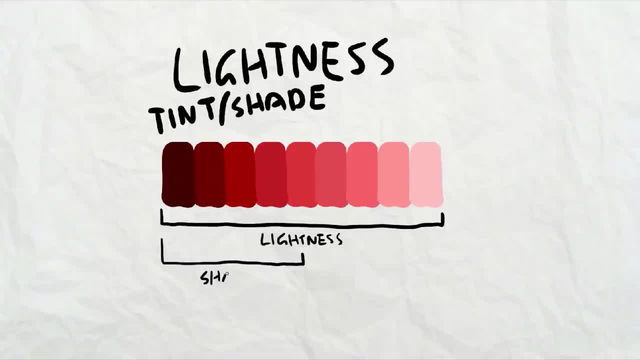 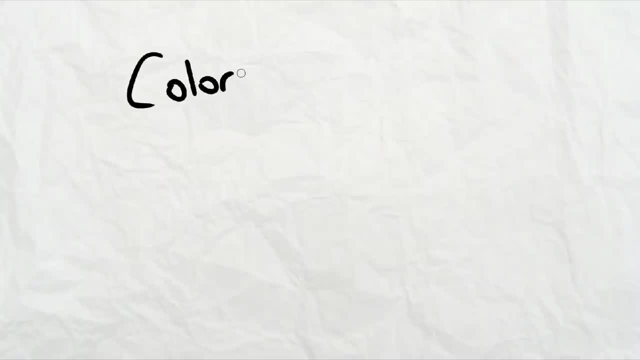 so you can sort of use a general term to call it lightness or brightness of the color. or if you just make it darker it's called a shade, if you make it lighter, it's called a tint. so next up is color groups. this is probably one of the more confusing parts of color theory. I'll try to make. 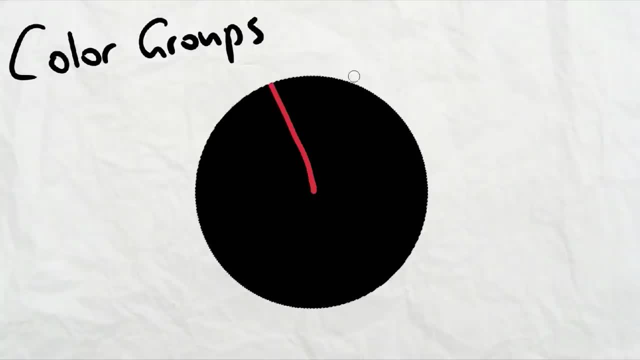 it pretty straightforward for you all, because it's pretty simple once you understand it. so I'm going to draw a little color wheel here and I'm basically going to show how different colors relate to each other. essentially, color groups are basically the same colors, but they're different colors, so I'm 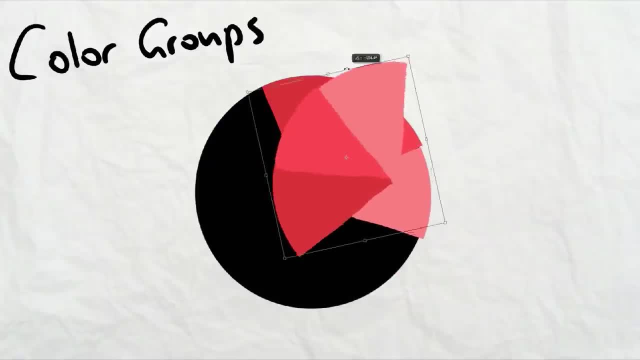 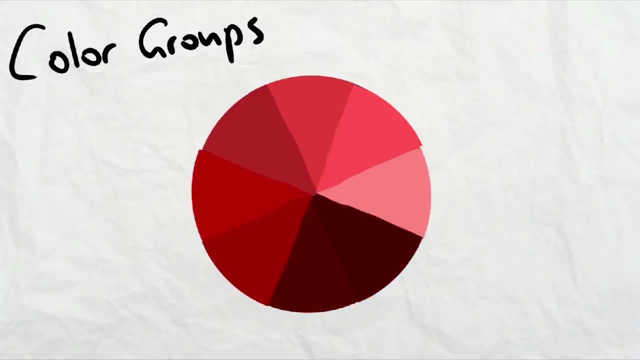 basically just color schemes. you could use these color screens for an artwork or for a painting or anything you're creating. it's just a way that colors can look cool together and sort of interact with each other. so what I've drawn right here is a monochromatic color scheme. it's essentially what. 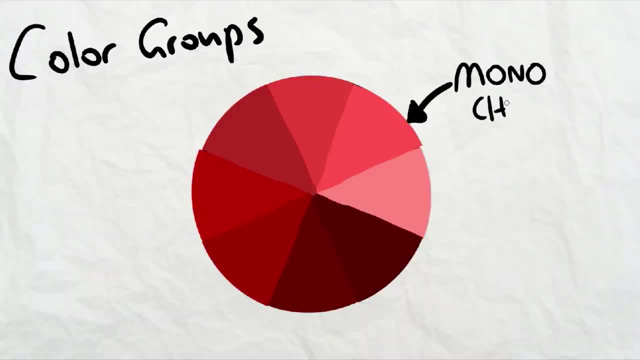 we just talked about, with tints and shades, except only one color. so if I was to make a painting just out of reds and nothing else, that would be a monochrome color scheme, and it's one type of color scheme that we can use. the next is analogous, or analog for short, analog is a color scheme that 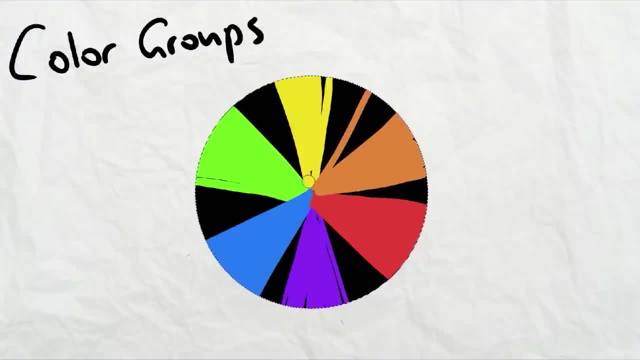 I guess you could say: and this is basically what color is next to another color. so I'm going to draw a little color wheel here and this sort of analog color scheme is basically picking three colors on this color wheel and they all just need to sit next to each other. so if I draw some little lines, 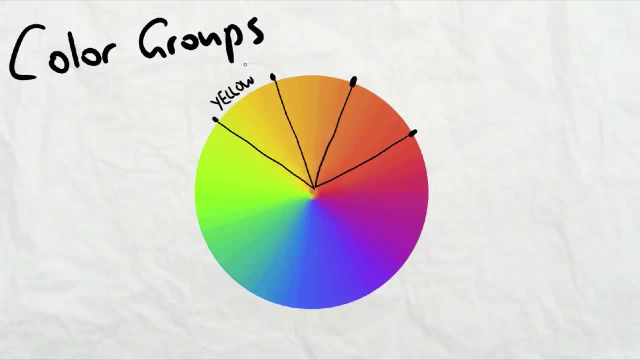 here. let's say we're going to pick yellow and then we'll pick orange- in the middle, if we spell it right- and then we'll pick red too, and that's an analogous color scheme. we've picked three colors and this can apply for any colors, so if I just rotate this over here and spin it around, it can. 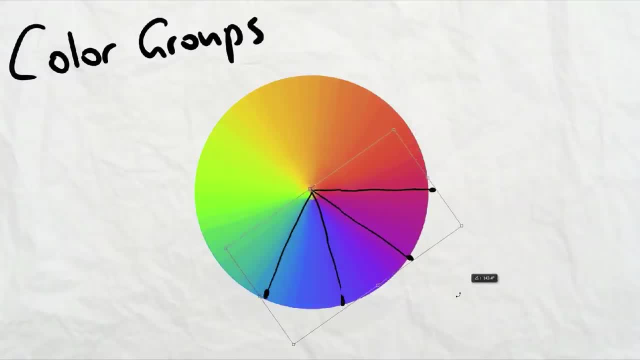 work for any colors. so I could pick a green, a yellow and an orange, I could pick a blue or purple and a red. they just need to sit next to each other in the color wheel. next is complementary. you'll probably hear this a lot in sort of art and design, and this is basically colors that are opposite. 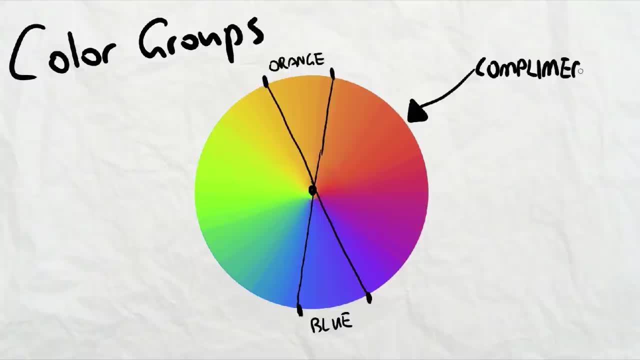 each other in the color wheel. uh, you've probably seen a lot of movie posters love to use the colors orange and blue. they're complementary colors. they work really good together, same with green, red and yellow and purple. so basically it doesn't matter what the colors are, they just need to be. 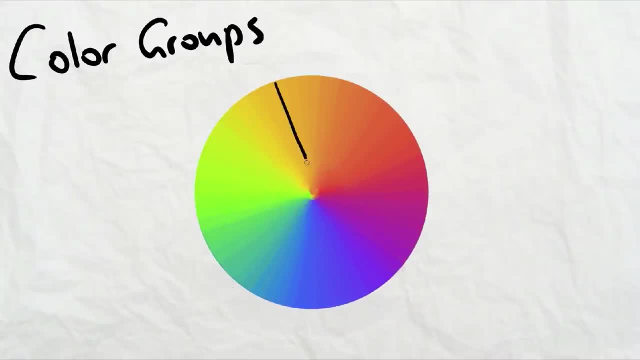 opposite each other in the color wheel and they are complementary colors. the next color group we're going to talk about is triadic, so this is essentially making a triangle on the color wheel. uh, so if we pick orange, green and purple, make a little triangle. that's a triadic color scheme. 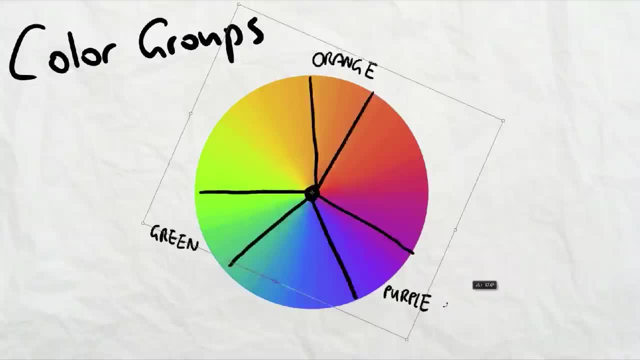 they all sit at a triangle's point away from each other. so if you just made a perfect triangle anywhere in the color wheel, as long as they all sit evenly, that's a triadic color scheme. there's a lot more color schemes than these ones I've just listed here, though. 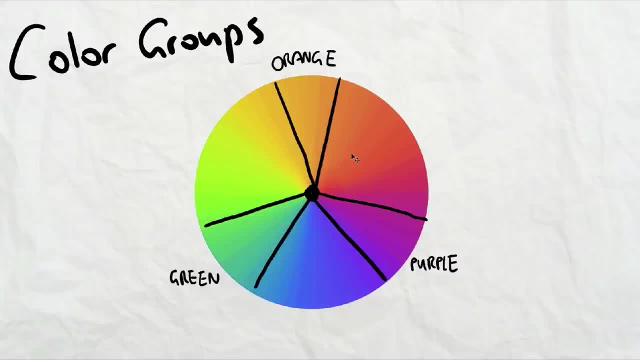 these are sort of the core, fundamental color schemes or color groups and, to be completely honest, you don't always use all those other color groups. it's more or less Theory. you do apply it in, like when you're actually creating your artwork, though I can say, as an artist who works in the 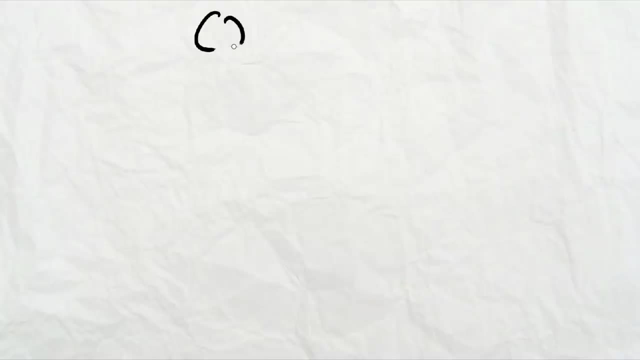 field. I don't often actually refer to the color groups. and the next part, and one of the most important parts, is the meaning behind colors. so a lot of people don't actually understand a lot of colors are picked for very specific reasons and each color actually has a meaning. 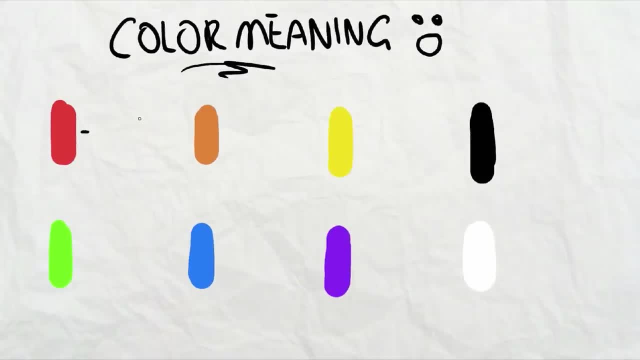 behind it and it gives off a certain emotion. whether you like it or not, each color actually does have emotion and meaning behind it. for anybody it's not subjective. um, all of these colors do actually give off a bodily sort of emotion and an impact that we don't actually. 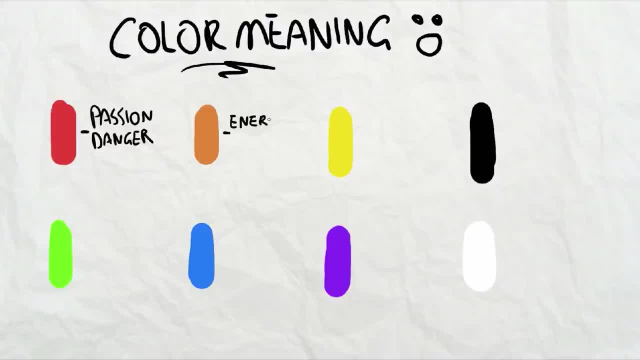 realize so. red is most commonly associated with passion and danger and fire and heat. that's why stop signs are red, uh. orange is often associated with energy and creativity. yellow is sort of happiness, joyfulness, energy, being active. you'll see this a lot with advertising people using these colors as well. black sort of 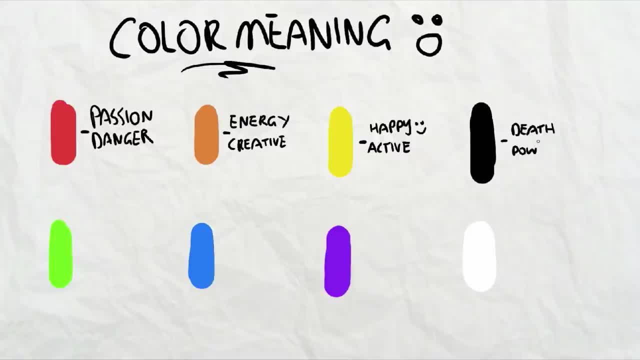 obvious. it's really associated with death and also power as well. green most commonly associated with nature, as well as healing and medicine. you see a lot of health symbols in games. be green for this reason. blue is also a calming color. see a lot of hospitals have a lot of health symbols in games. be green for this reason. um, it's also associated with 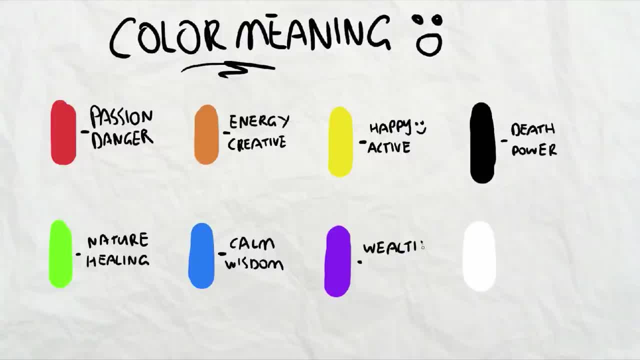 wisdom. purple is often associated with wealth. actually, the reason this is is because the color purple- uh, the actual dye- was a lot harder to create and make a few hundred years ago, so it was often only sort of worn by kings and queens and Royals. so that's why it's sort of associated. 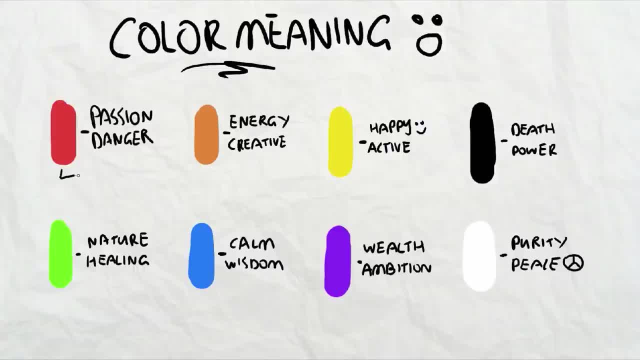 with that, and white is obviously known as sort of purity and peace, basically the opposite of black. we also have warm and cool colors. green is somewhat of a neutral color, but let's just say it's cool. so obviously red, your orange, yellow are all somewhat warm colors. blue, purple and green are somewhat cool colors and you can 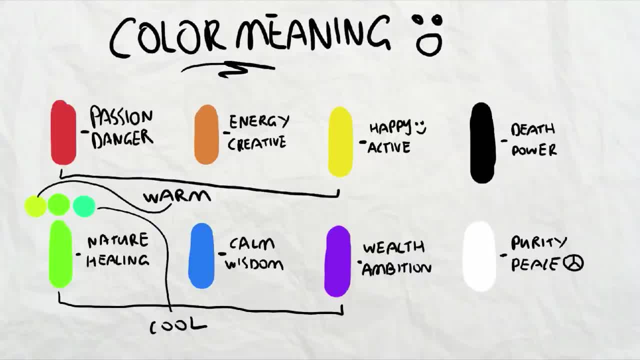 also make any color on a color wheel warm or cool. so I've duplicated the green here so you can see the dot on the left of the green has a bit more yellow added to it, so it's a bit more warm. and then the dot to the right of the green dot has a bit more blue added to it, so it's a bit more of a 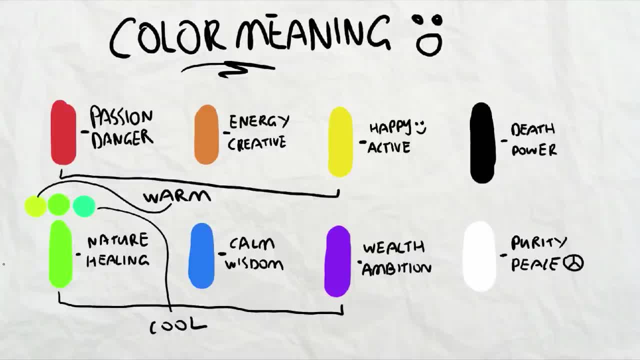 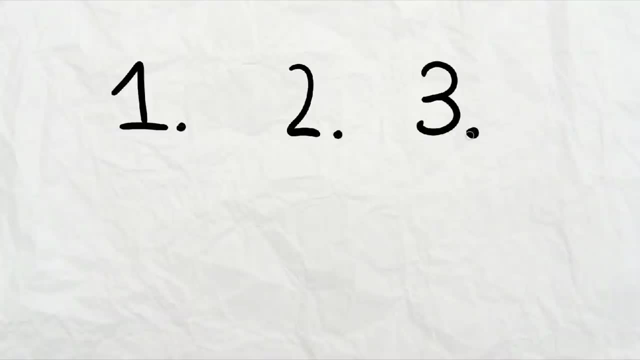 turquoisey color and that's more of a cool color. so if people refer to warm or cool colors, it's essentially how much yellow or how much blue has been added to a color. so yellow being warm, blue being cold. so next I have a little test for everybody watching, uh. so I want you to go through this with me, so I'm going. 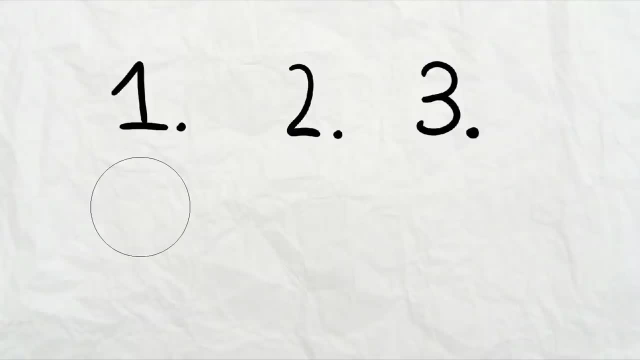 to draw three blue dots on my screen right now and I'd like to basically get your idea of what's happened to these blue dots. so I've got one, and I've got two, and I've got three. so on the first dot, I'm going to change something about this dot and I want you to write in the comments what I've. 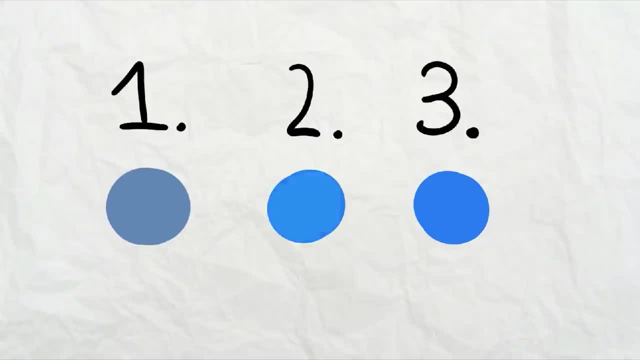 changed about that dot. the second dot: I'm going to change something about this dot as well. I want you to let me know what did I change. what type of color, sort of meaning did I change? and the third dot: I'm actually going to create a color scheme and I want you to tell me what color scheme or color group.